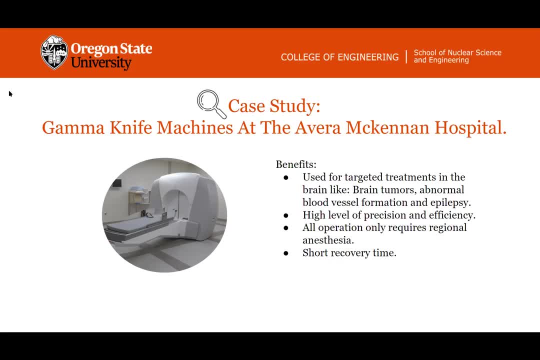 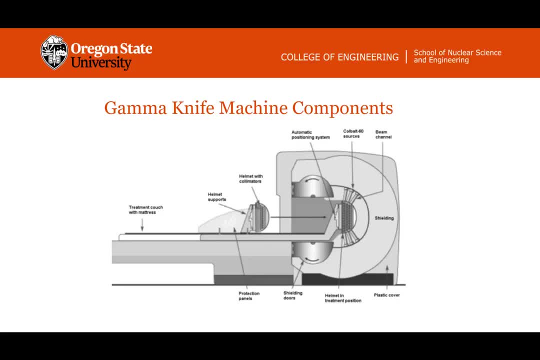 Decommissioning also ensures that work is done to restore the environment after a facility is closed down. Decommissioning also ensures that work is done to restore the environment after a facility is closed down, the millimeter allowing for extremely precise applications of the radiation, allowing it to 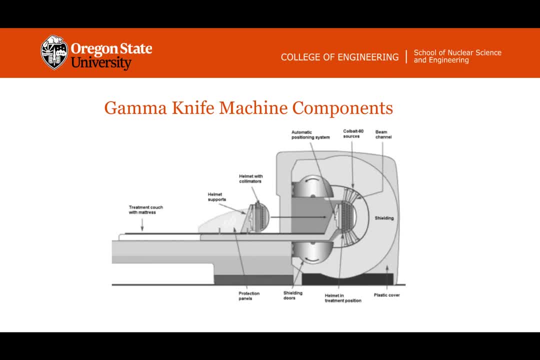 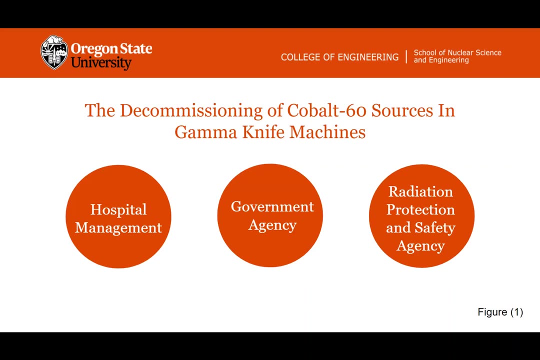 target very non-conventional geometries within the head in multiple doses or to contact very small targets without affecting the surrounding tissue. So the way we decided to break up the project is to look at the three different agencies or groups that would be involved in a decommissioning. 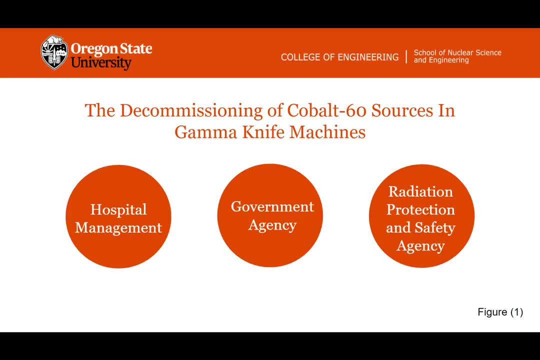 process. We wanted to look at the hospital side, managing the decommissioning and coordinating with both the government and third parties. We wanted to look at the government side of the project and the regulatory oversight that goes into a decommissioning project And we wanted to look at the hands-on radiation protection and safety side where a company comes. 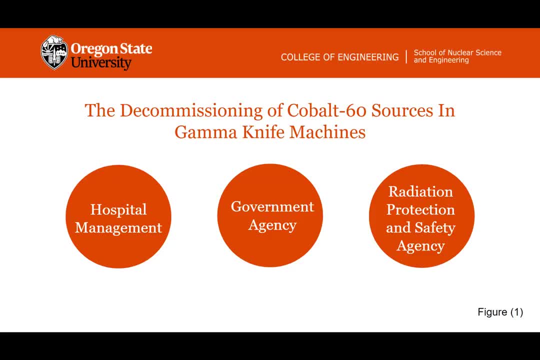 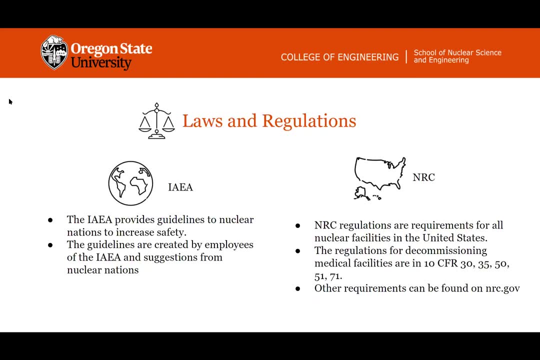 in, sets up the appropriate machinery and equipment and removes the sources safely. The primary sources of radiation are the radiation and the decommissioning. The primary sources of radiation are the radiation and the decommissioning, The primary sources of the regulations and guidelines followed for nuclear decommissioning. 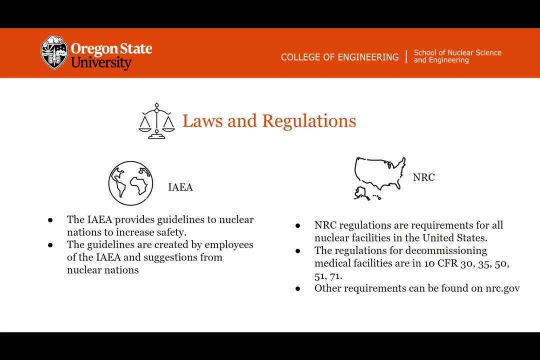 are from the IAEA, the International Atomic Energy Agency, and the NRC, the Nuclear Regulatory Commission. The IAEA is a UN-associated agency that works with the nuclear nations around the world to increase safety for peaceful nuclear activities. They produce guidelines that they recommend nations base their regulations on. The NRC is the private. 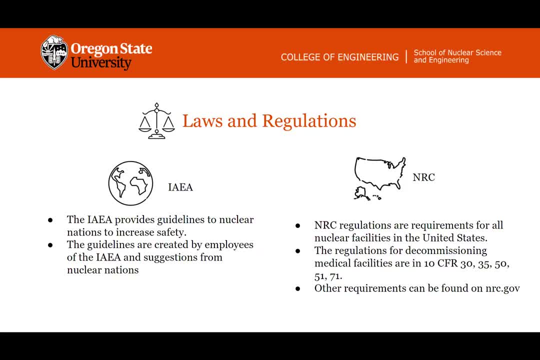 nuclear regulator for the United States and has most of the relevant regulations in the Code of Federal Regulations. The most relevant regulations can be found in 10 CFR, 30,, 35,, 50,, 51, and 71,, with most of the remaining requirements being on the NRC website. 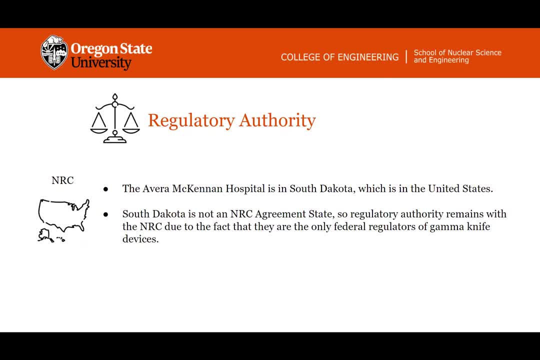 Before decommissioning, it is necessary to understand who has regulatory authority over the process, Because the Avera-McKinnon Hospital is in South Dakota, which is not an NRC agreement state, we know that the NRC is the primary. 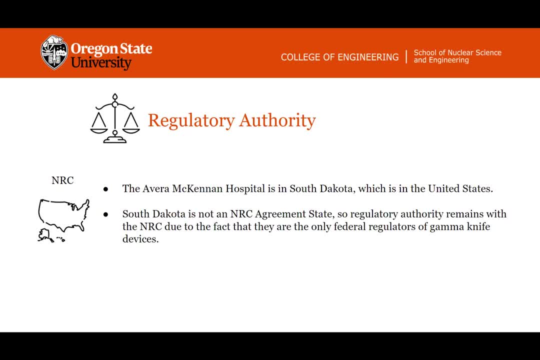 regulator and the process will have very limited state involvement. Additionally, because we are focusing on the Gamma Knife machine at the Avera-McKinnon Hospital and the NRC is the only government agency that regulates Gamma Knife devices, the only relevant regulatory authority is the NRC. 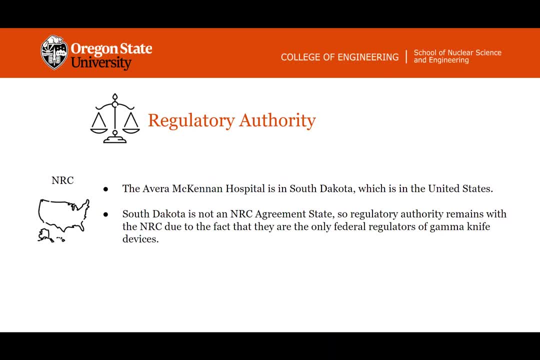 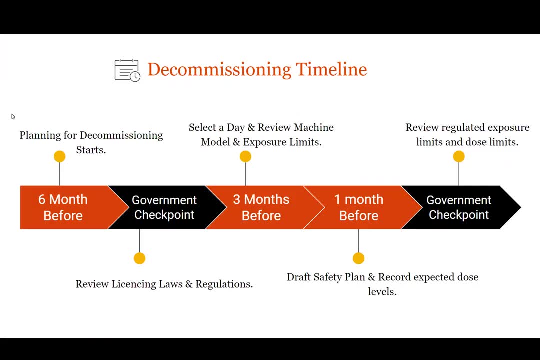 The following timeline breaks down the decommissioning operation by months, six months, three months and one month. During the six-month mark, the hospital personnel will start and initiate the planning stage of the decommissioning by contacting the radiation protection and safety agency, the NRC, and the NRC. 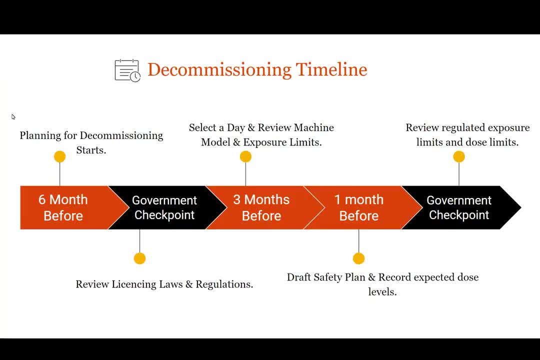 The NRC will then begin the decommissioning operation. The NRC will then begin the decommissioning operation. The employees and staff will then begin to focus on the decommissioning operation at the NRC and what needs to be done. The emergency concepting quickly start to expand. 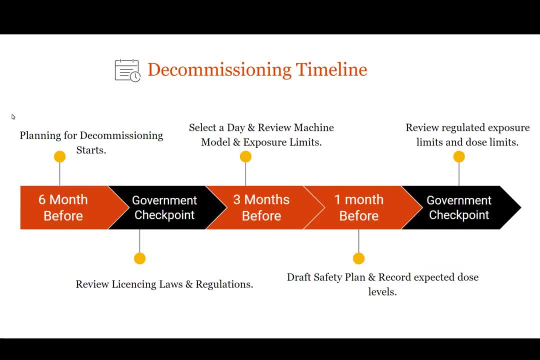 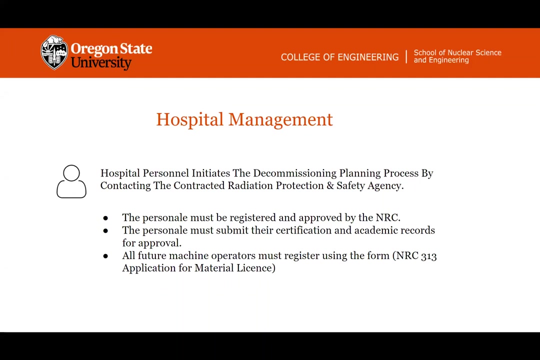 in the surveillance- нова's lower. there'll be a lot of safety planning and recording expected dose levels At each point. there'll be a lot of government regulation reviews and to make sure that everything is going within regulatory guidelines. So the first step in the hospital management, as I've mentioned, 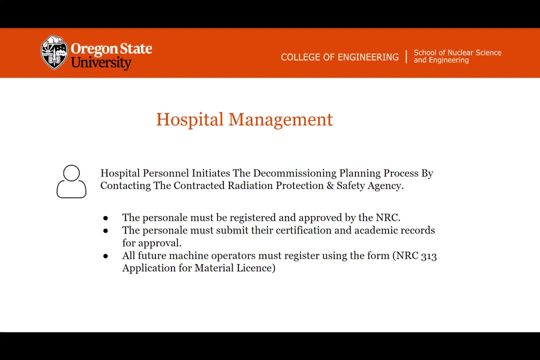 hospital personnel will initiate the decommissioning planning process by contacting the contracted radiation protection and safety agency. What we need to know about this hospital personnel is that they must be registered and approved by the NRC. The personnel will submit their certification and academic records for approval before this whole process starts. 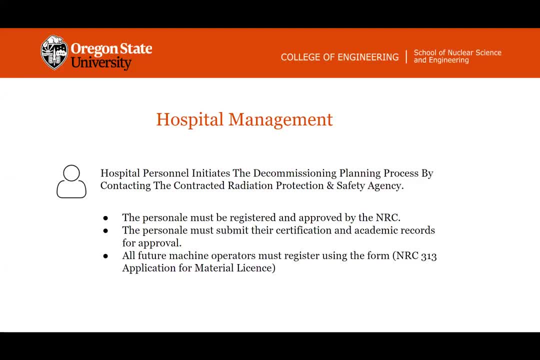 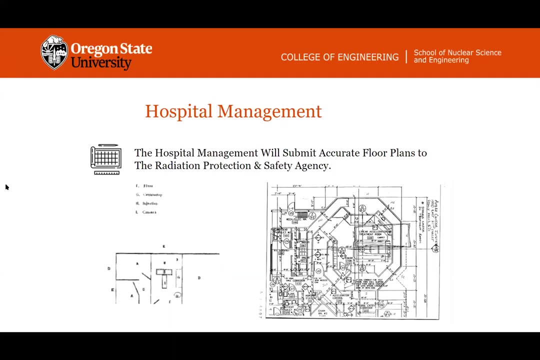 And in the future, any machine operators will have to register using the same process through the NRC, using the application for material license. The second step will be submitting accurate floor plans to the radiation protection agency. This will help both the hospital and the radiation protection agency to plan an exit strategy or calculate accurate dose expected. 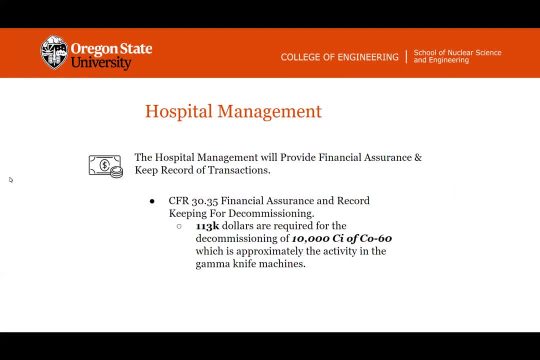 dose. The hospital management will provide financial assurance and keep record of all transactions. This is also following regulation from the NRC SFR 3035: financial assurance and record keeping. for decommissioning, It is required by law that the hospital will put aside $113,000. 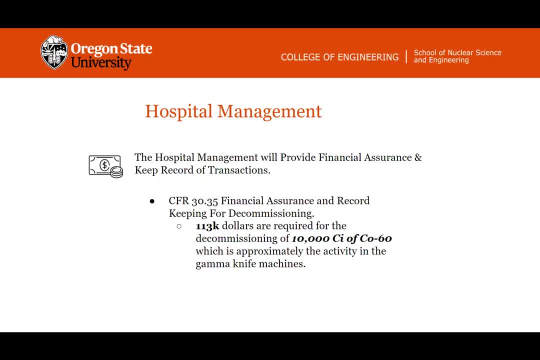 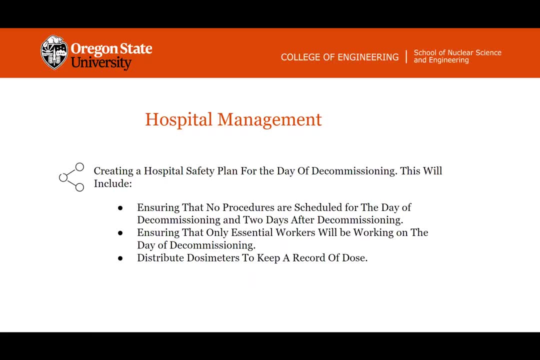 just for the decommissioning operation of those cobalt 60 sources. and, lastly, the hospital will create a safety plan for the decommissioning and this will include ensuring that no procedures are scheduled for the day of decommissioning and two days after the decommissioning is completed. 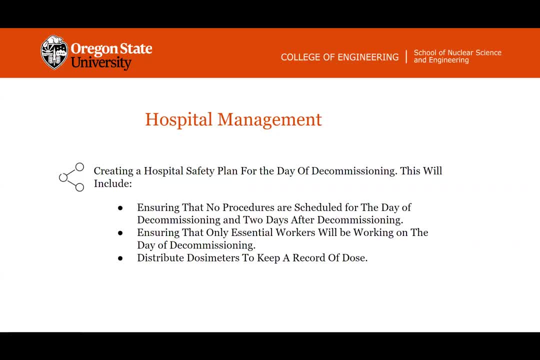 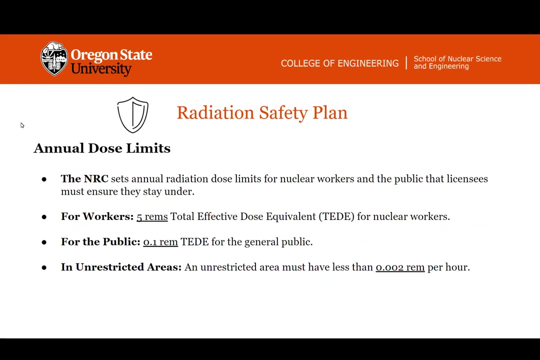 ensuring that only essential workers will be working on the day of decommissioning and distributing dosimeters. to keep a record of dose, Randy. Now regarding the actual radiation safety plan, there are a couple of pieces of regulation that we need to make sure that we're staying within so that we're keeping our workers and the general 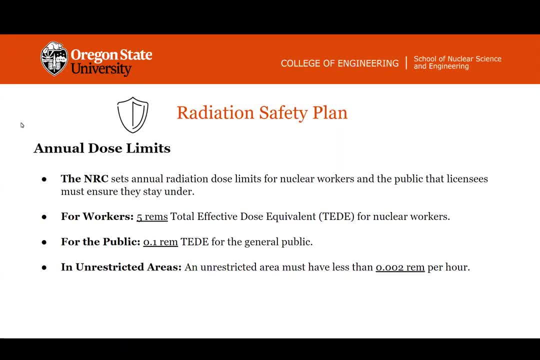 public safe. The NRC has set annual radiation dose limits- uh that are both different for nuclear workers and the public- that the licensee has to make sure that we stay under. for the workers That means 5 rems total, effective dose equivalent- and for the public it's 0.1 rems total. 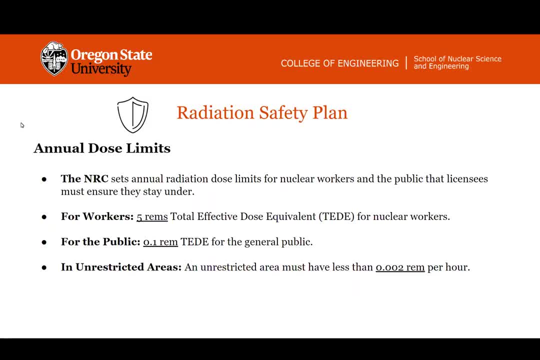 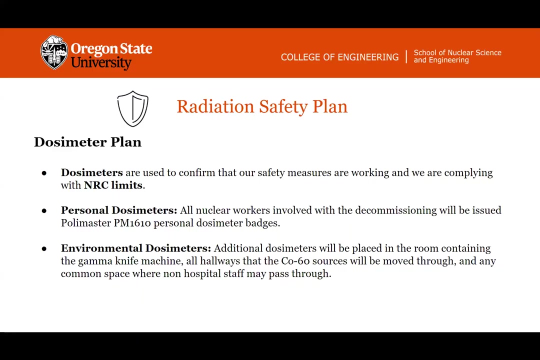 effective dose equivalent. And in any unrestricted area or an area where any random person could walk through unrestricted without being stopped, there has to be a dose rate of less than two thousandths of a rem per hour. Next slide. So how we're going to accomplish this is through the use of dosimeters. Now, dosimeters are devices. 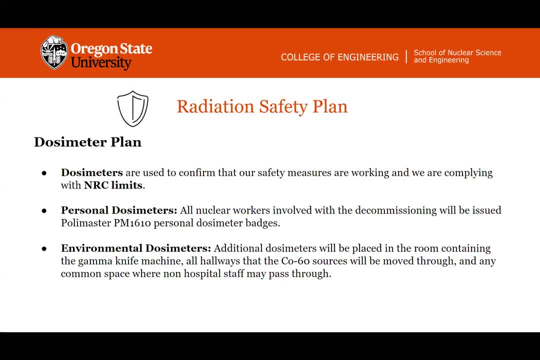 that can be worn or placed in an area to measure the exposure to radiation in that area or on that person. Dosimeters, however, are not what's keeping you safe from radiation. All a dosimeter does is it sees how much radiation you've received, and this is important in making sure that our safety. 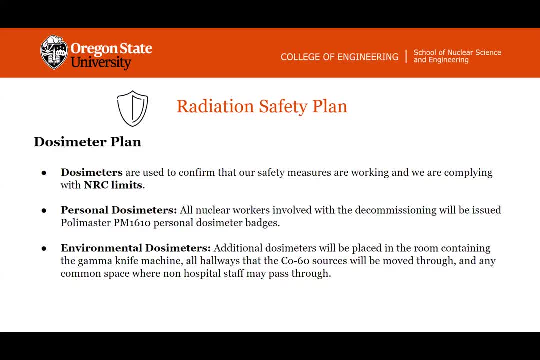 plans. our shielding, the time we spend around radiation and how far away we keep people from the radiation is actually working and keeping the exposure to radiation low for those individuals. So we'll be handing out personal dosimeters to all nuclear workers that are involved with decommissioning directly. 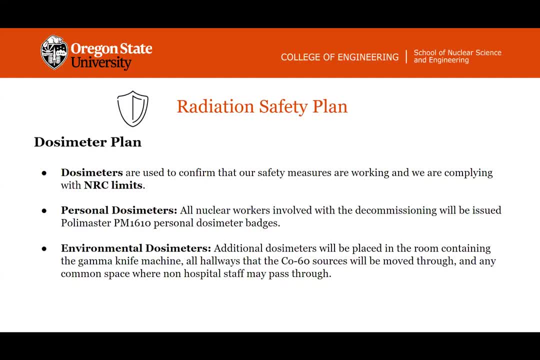 These dosimeters will be Polymaster PM 1610 personal dosimeter badges that can be worn on their uniforms. We'll also be using similar dosimeters that will be placed in the area around the decommissioning. This includes the room of the Gamma Knife Machine on the Gamma Knife. 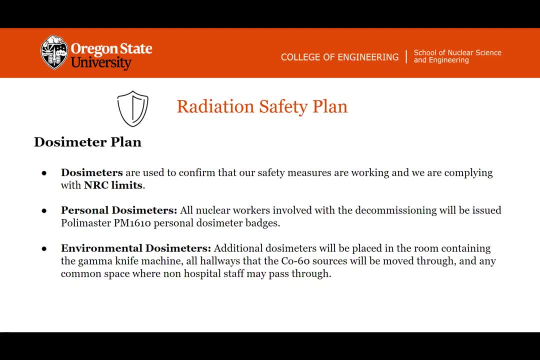 Machine and all of the hallways and corridors that the Cobalt-60 sources will be moved through during the decommissioning process. We'll also be placing these dosimeters around any common space where non-hospital staff may pass through, making sure that these unrestricted areas' dose stays low. 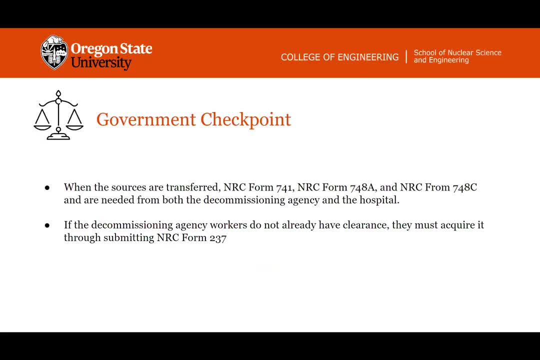 Before the sources are transferred, there are a few government requirements that must be met. Among them is the requirement for the hospital and decommissioning agency to complete NRC Forms 741,, 748A and 748C, which are used for the purposes of tracking sources. 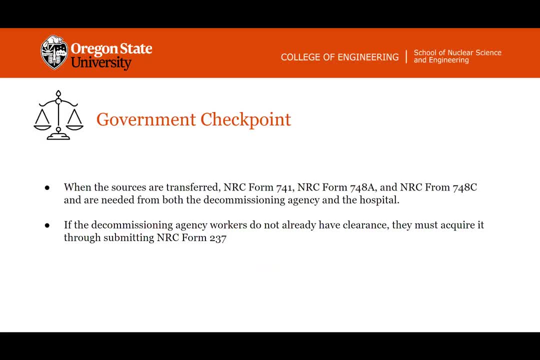 Form 741 is a form to track the sources for the IAEA, and Forms 748A and 748C are for the NRC's records. Additionally, if the decommissioning workers do not already have clearance to work on the Gamma Knife device, 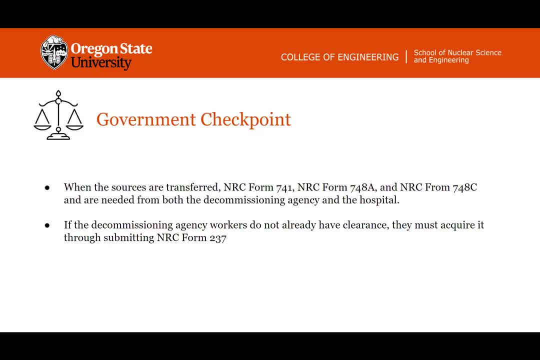 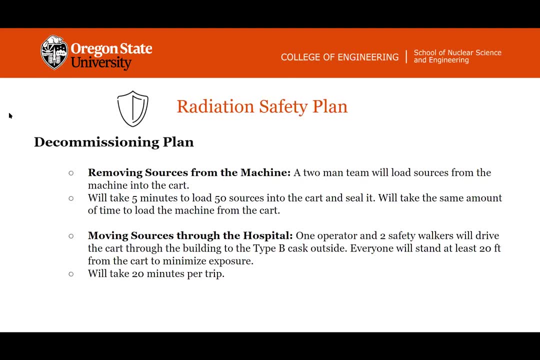 they must request and receive authorization. They must request and receive authorization from the NRC by submitting NRC Form 237.. Next slide Now, regarding the actual plan for our workers. what we're going to be having them doing is removing the sources from the machine. 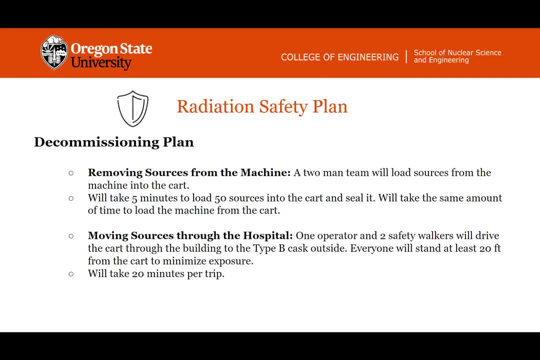 and then moving them through the hospital and placing them in a cask outside for transportation. A two-man team will work on loading the sources from the machine into a cart that is shielded and then moving that cart through the hospital. It'll take five minutes. 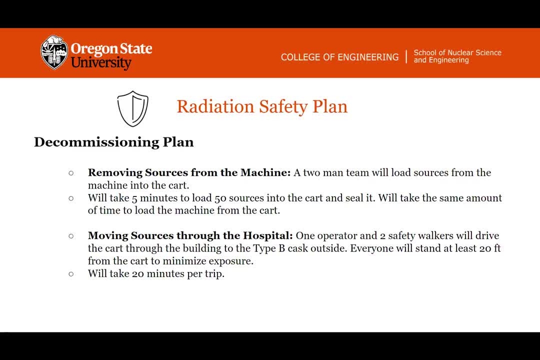 It'll take five minutes to load 50 sources into the cart and seal it and it'll take four trips to get all 192 sources in the cart. And it will take the same amount of time to load the machine, to load the cart from the machine into the cask and vice versa. 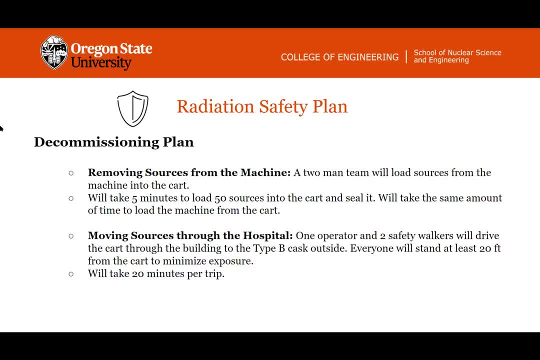 Moving the cart through the hospital. one operator and two safety walkers will drive the cart through the building to the Type B cask that's outside. Everyone will be required to stand at least 20 feet away from the cart to minimize this exposure In each trip. 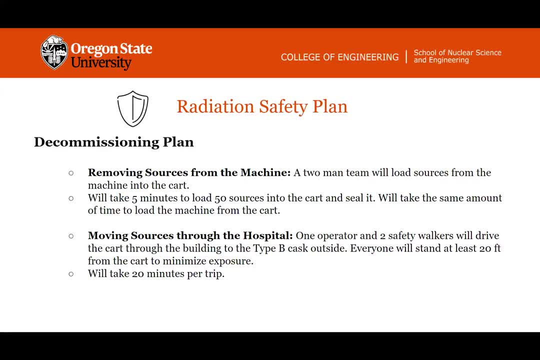 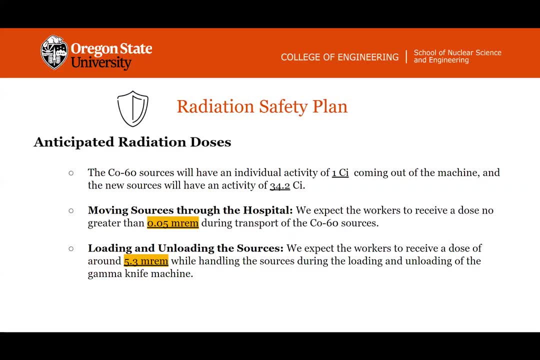 it'll take roughly 20 minutes to get the cart from the inside of the hospital to the outside. Looking at how much radiation we expect our workers to receive, we first look at how active the sources are. Now when we're decommissioning these Cobalt-60 sources, their activity is going to be very low. 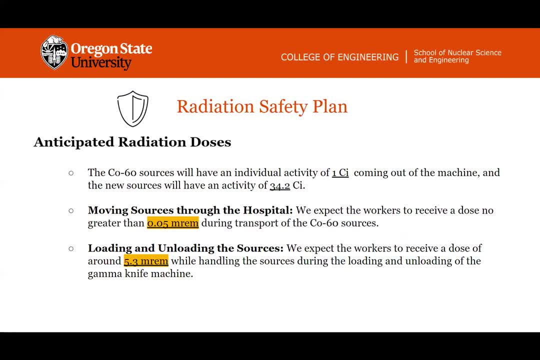 So we anticipate an individual activity of each source of one curie coming out of the machine, and the new sources that we will be bringing to the facility will have an activity of 35. 44.2 curies, which is much higher. We expect the workers to receive a dose of no greater than 0.05. 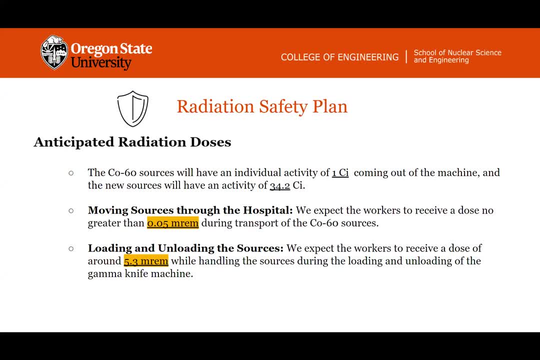 millirems during the transportation of the Cobalt-60 sources. This is moving them from the machine to the truck outside and from the truck to the machine inside, And we expect no more than 5.3 millirems of radiation dose for our nuclear workers while they're actually handling the. 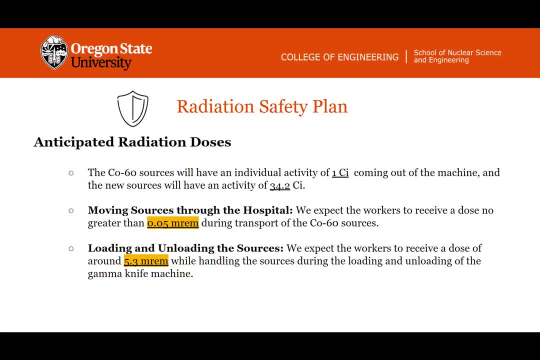 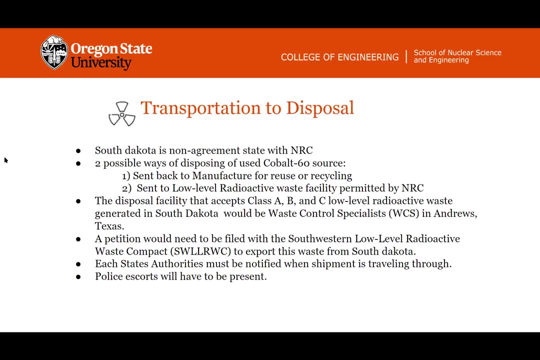 sources directly moving them from the various containment systems and into the machine Total. we're expecting less than 6 millirems per worker and less than 0.05 millirems for anyone in the general public. Next slide, Once the used Cobalt-60 sources have safely made it out of the facility. 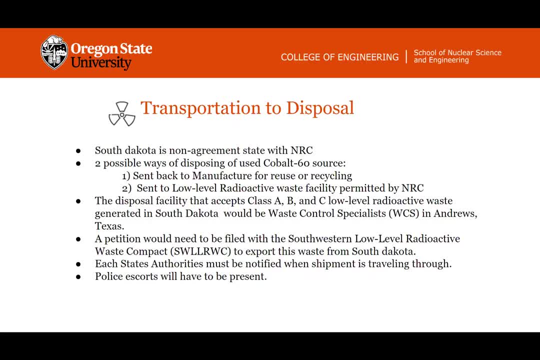 it's time for transportation to disposal. South Dakota is a non-agreement state with the NRC, meaning that the NRC has regulatory authority for radioactive license in South Dakota. Two possible ways of disposing of the used Cobalt-60 sources include one being sent back to the manufacturer. 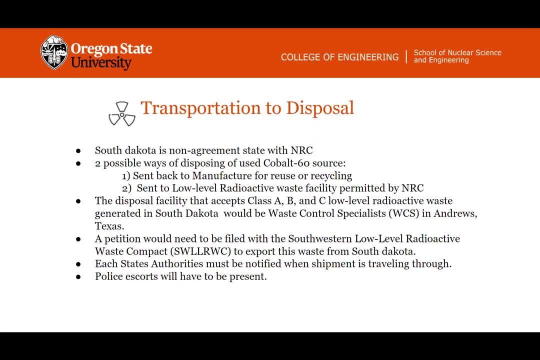 for reuse or recycling and two sent to a low-level radioactive waste facility permitted by the NRC. For this case, we will be sending it to a low-level radioactive waste facility. The facility that accepts Class A, B and C low-level radioactive waste generated in South Dakota would 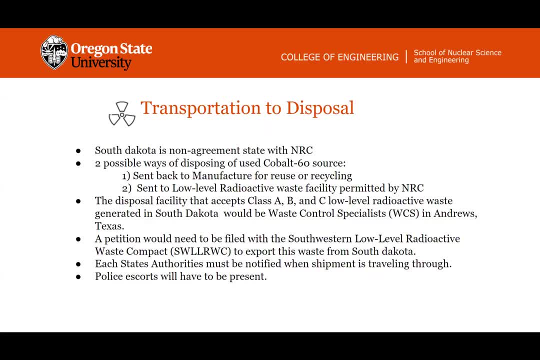 be known as the Cobalt-60.. The NRC has regulatory authority for radioactive license. in South Dakota, The NRC is known as a State of Public Safety. The NRC is known as Waste Control Specialist, located in Andrews, Texas. In order to get the sources there, a petition would need to be filed with the. 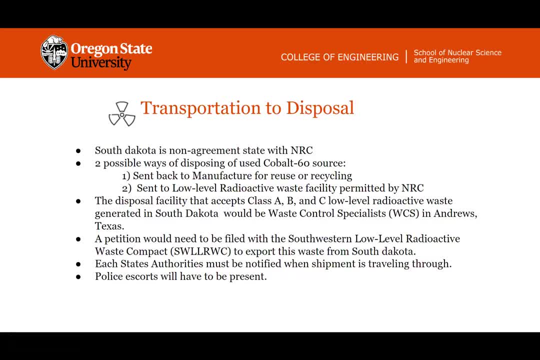 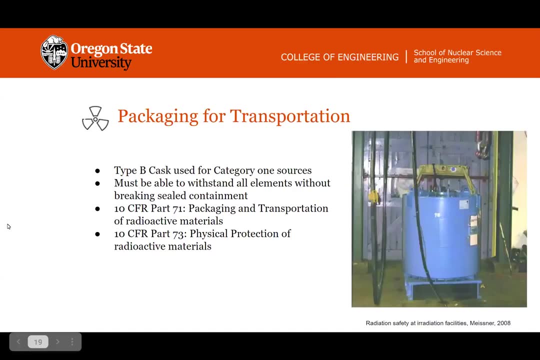 Southwestern Low-Level Radioactive Waste Compact. in order to export this waste from South Dakota, Each state's authorities must be notified when a shipment is traveling through, and police escort will have to be present during the transportation. Next slide: Packaging for transportation. The used Cobalt-60 sources will then be placed in a non-agreement facility. which will be used as a storage. ok, There are specific rules in place for transportation. The used Cobalt-60 sources will then be placed in a sewage tank and these will be used to causes waste and waste disposal, and they will be used for transportation In addition to the use of the waste control specialists. 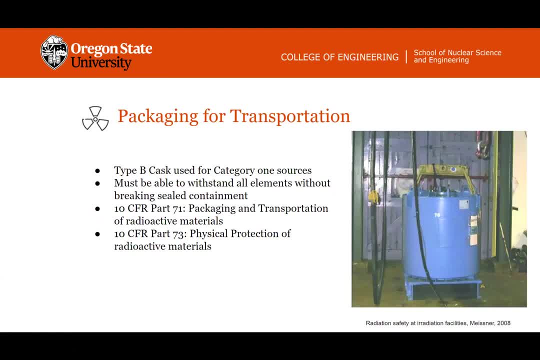 cobalt 60 sources will then be placed in a type b cast used for category one sources and must be able to withstand all elements without breaking sealed containment. this is tested through a number of tests that include a 30 foot free fall drop, a 40 inch drop on a steel rod and heating the package. 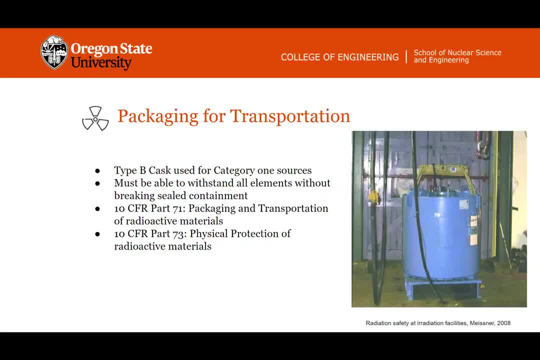 up close to a thousand degrees for 30 minutes and finally an immersion in water 15 feet down for 30 minutes. this ensures the containment abilities of the package. 10 cfr part 71- packaging and transportation of radioactive materials, along with 10 cfr- part 73- physical protection of. 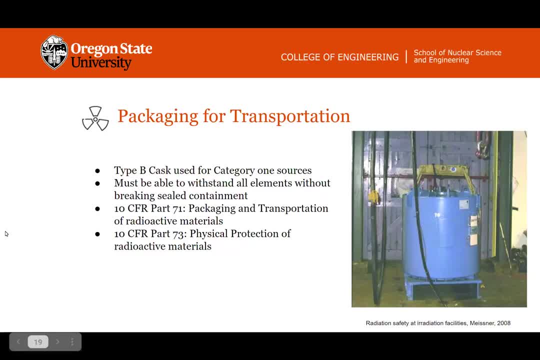 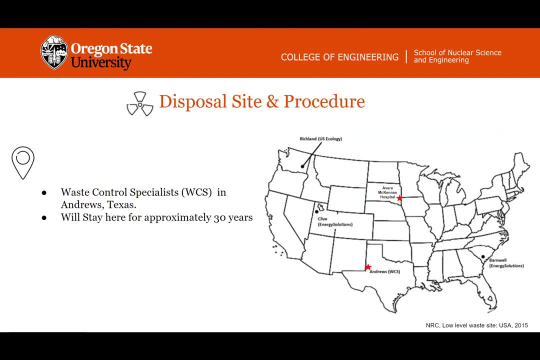 radioactive materials are very important during transportation. next slide: the waste control specialist in andrews, texas, is located at that red star, the southern star in texas, and our hospital is also located in south dakota, on the other, the most northern star, the cobalt 60. once it reaches this point, will be placed underground, where it will be state. 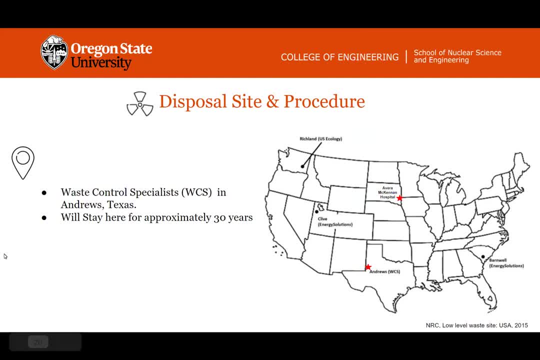 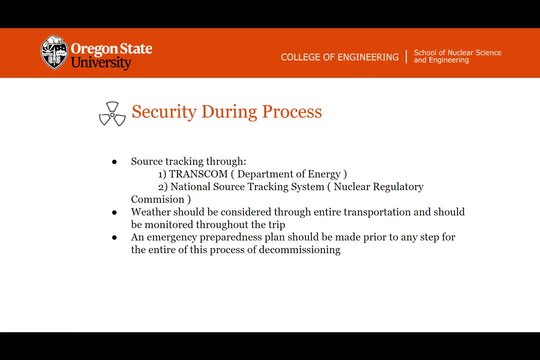 will where it will stay for approximately 30 years. next slide uh security. during the process. there's source tracking through transcom, which is put on by the department energy and is used by doe shippers and a couple other agencies during transportation, and also the national source. 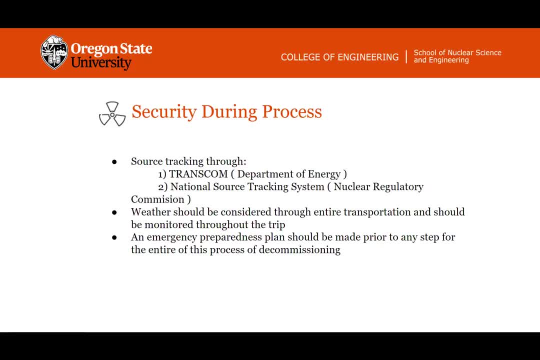 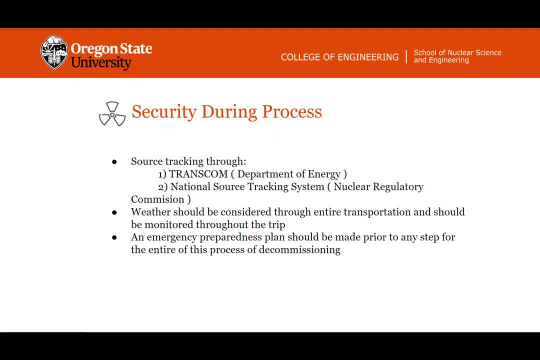 Weather should be considered through the entire transportation and should be monitored throughout the trip to ensure that there is no bad weather that we run into. An emergency preparedness plan should be made prior to any step of transportation for the entirety or the entirety of this process. 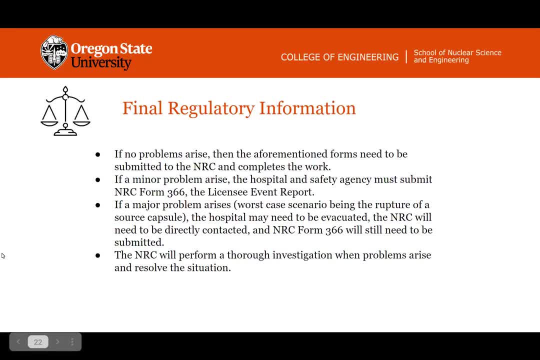 of decommissioning. If the decommissioning encounters no problems, then the work is complete once the necessary forms have been sent to the NRC. If a minor problem arises that does not require immediate intervention, then the hospital and decommissioning agency need to submit.